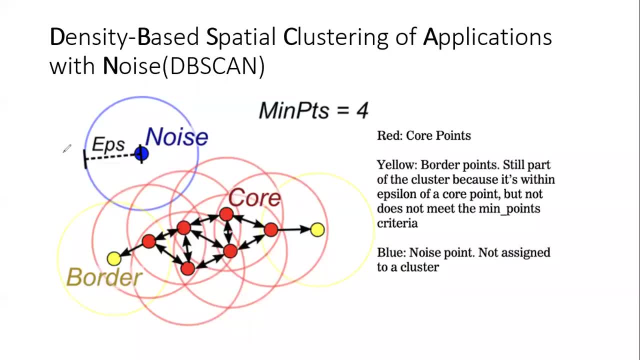 Hello all. Today we will be discussing about DB scan algorithm. So the full form of DB scan is something called as density based spatial clustering or application with noise. Don't worry about so big full form of this particular topic, but it is a very easy topic to understand. machine. 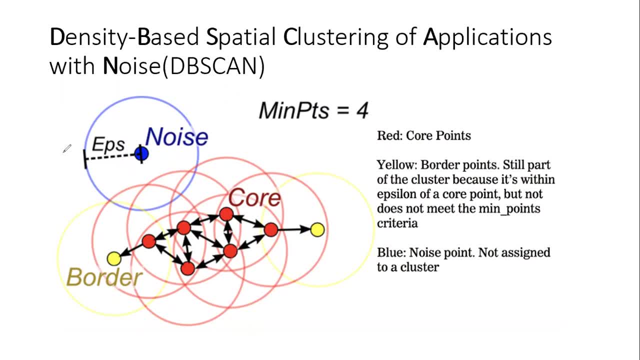 learning algorithm. So DB scan algorithm is one of the most better unsupervised machine learning technique, which sometimes performs better than k-means clustering and high-clean clustering. but it has its own advantages and disadvantages, which we'll be discussing at the last in this particular video. So make sure you watch this particular video till the end, because I've 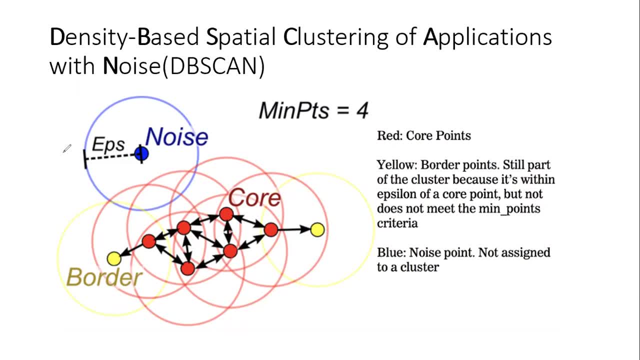 explained the both intuition part and the implementation part with the help of Python and Scalern, and how you can actually implement this particular algorithm. To begin with, guys, the most important thing over here is that it has four important components. One is something called as epsilon. 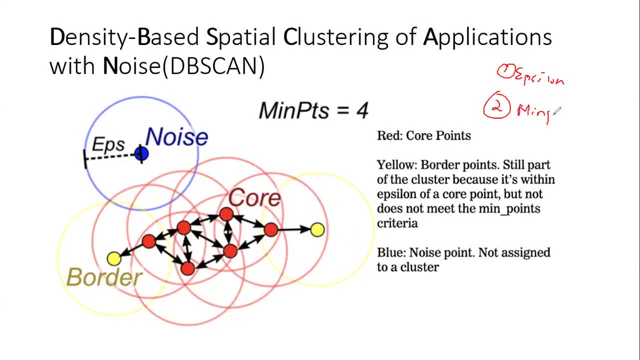 The second component is something called as minimum points, Then you have something called as core points, Then you have something called as border points and you have something called as noise points. So, as you know, that DB scan is an unsupervised machine learning technique. So 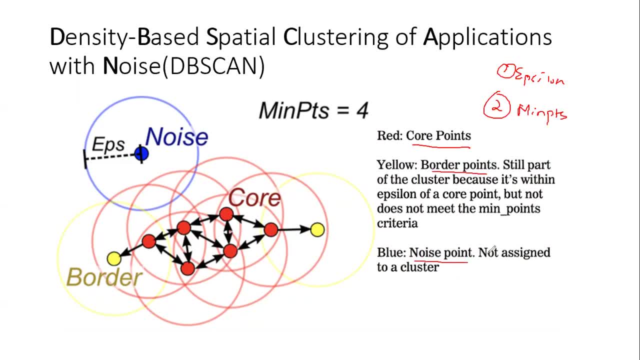 basically an unsupervised machine learning technique. it happens in such a way that it works in such a way that whenever we have some data points populated in a particular graph, it may be two dimensional or three dimension. What we do in unsupervised machine learning technique is: 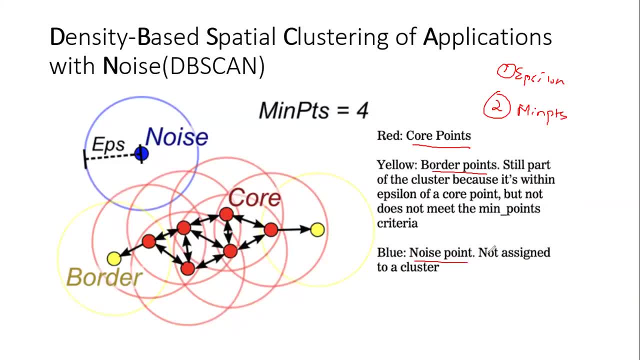 that we try to make up clusters. You know clusters helps you to find out the most similar points in our distribution and, based on that particular clusters, you know whenever a new point comes, like for the next test data, whenever I get a new data and if I try to populate. 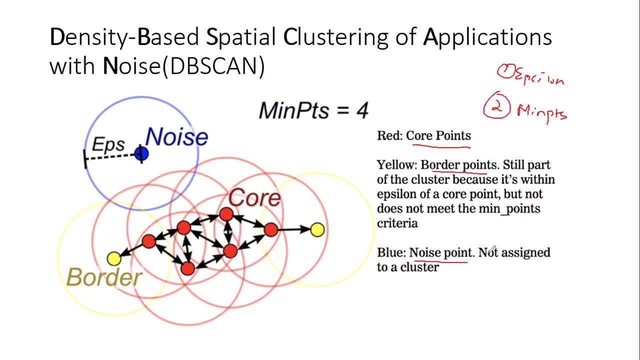 that point. whichever cluster that particular point will fall into, I'll consider that point falling into that particular group. So that is how a clustering algorithm works. I've already created videos on k-means clustering and hierarchical clustering. If you're interested, you can go. 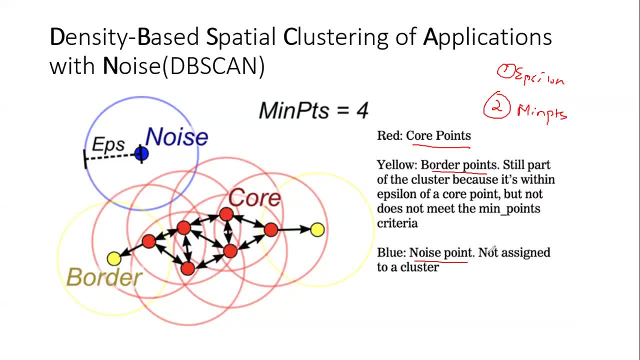 and have a look On to that, but we'll try to understand. how does density based spatial clustering works, and this is included with noise. Now, first of all, what we do is that we will be having initial points, So this will be basically all our points. So what we do is that we initially consider some epsilon. 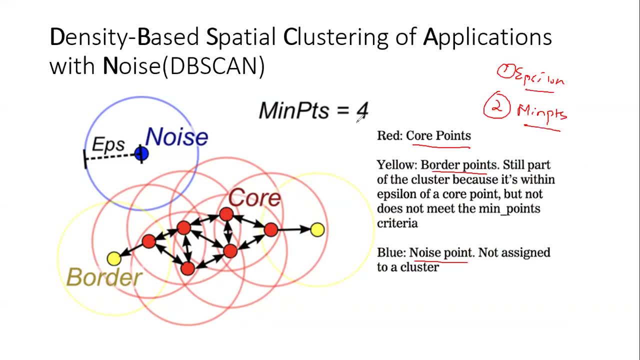 value and some minimum points value. So suppose if I'm considering over here as minimum value, minimum points as four, and suppose I say that my epsilon value is something like three, four, It depends on the distance. Now the epsilon value Indicates. very important thing that basically indicates is that suppose this is my point a, OK, 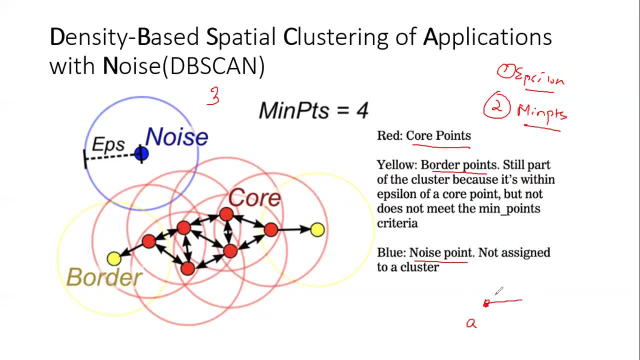 Now, what does epsilon indicates that I have to take the radius of that particular value of epsilon, OK, and then I have to create a circular path, that is, I have to create a circular boundary across it of that particular radius. So this is my radius, OK, Now, when I create this particular radius, the next, the next. 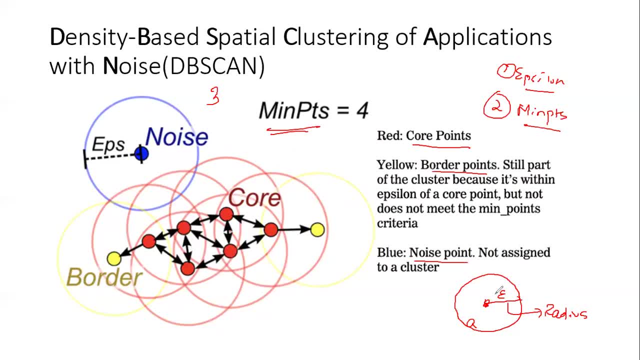 component, that is, minimum points, comes into existence. Now this epsilon will be based based on like within this point, I have to minimally considered, I mean, I have to consider a minimum number of points of four points in this. So if I, if I have four points like this, which is populated within, 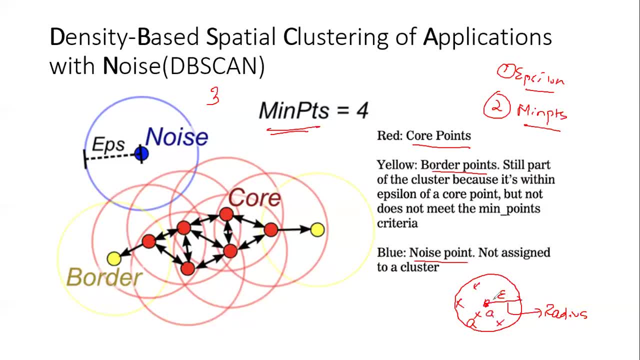 this, then what happens is that I will be considering this point a as my core point. So very important thing to understand: that to make a point considered as a core point, there should be two conditions. that has to be, you know that there should be two conditions that it has to follow. 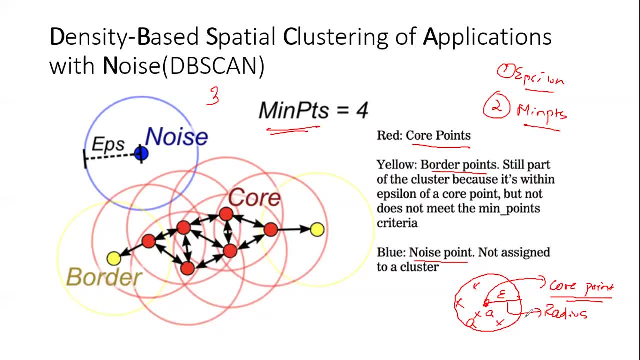 One is that I have to consider a boundary with the radius of epsilon value. Then the next thing is that I have also considered that the minimum number of points that fall within this boundary should be less than or equal to four, in this particular case, Right. 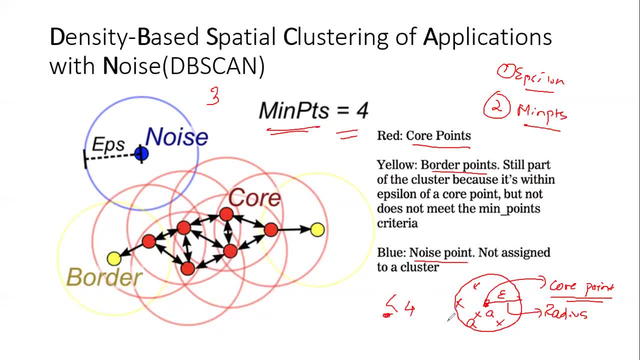 Sorry, it should be. at least four points should be following in this particular thing, Right? Or if it is greater than four point, it is well and good, but at least four points, you know. at least four points should be following in this particular boundary. Then only I'll be considering the. 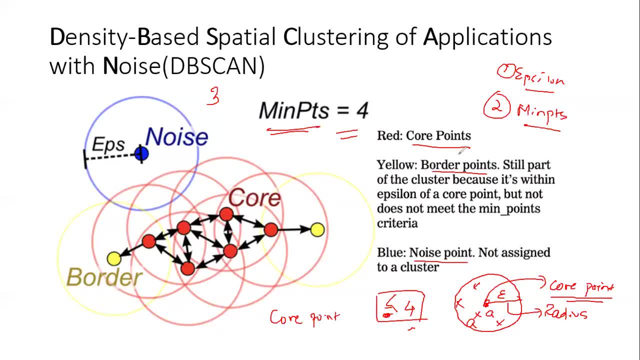 this a point as my core point. So my next component that I was discussing about is something called a score point. Now there is also something called as border point. a border point indicates something. Now suppose I have a point C. OK, Now I'll be using my epsilon value and creating. 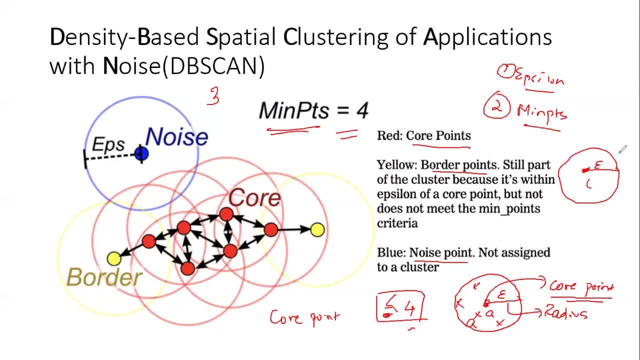 my epsilon value Right, I'll be creating that radius and with respect to that, I'll be creating my boundary. Now this particular C point. suppose it does not satisfy. the minimum points is equal to four. OK, It does not satisfy, this Minimum point is equal to four. But we have at least one core point present inside this particular boundary. 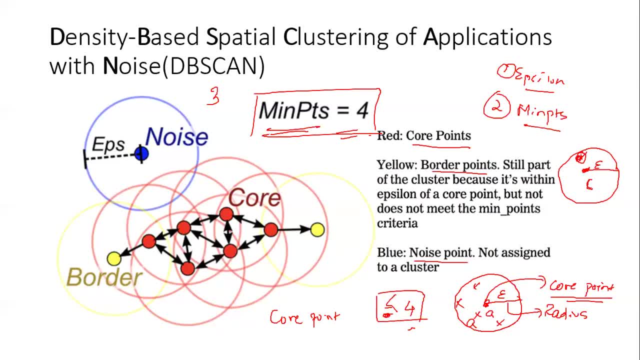 OK, Now just understand these guys. two condition: First of all, I have drawn the boundary with the help of epsilon. The second condition is that this minimum points is not getting fixed. That basically means I don't have that many minimum number of points that I've actually initialized in this. 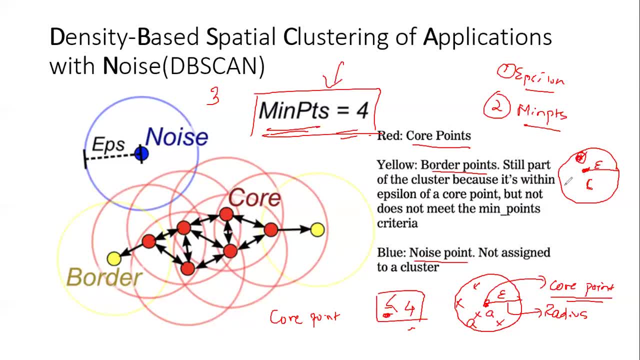 But I have one, at least one core boundary inside it. So when I have this one core boundary inside it, then this points Actually becomes a bound, border points, But this point actually become a border point. Now, three things, guys. First of all, we need to understand what is epsilon, with the help of epsilon and creating the boundary. 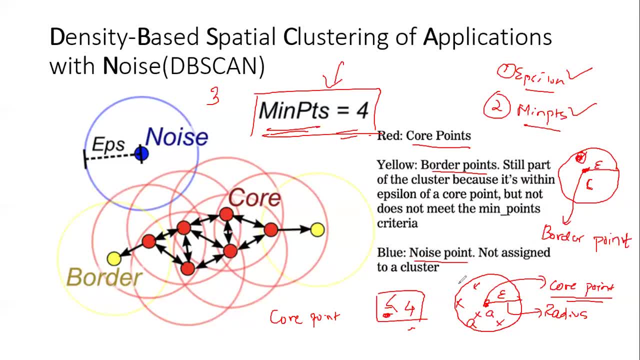 Second condition is that I have to consider that minimum number of points up has to be present within that boundary. Then only I'll be able to consider this point as my core point. OK, If it is not falling, Then what do we do? is that we consider another scenario wherein we consider that 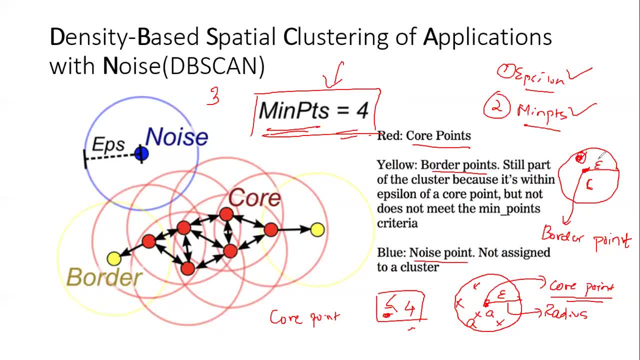 at least one core point should be falling inside this boundary. If one core points, four points basically means this kind of point- If it falls inside this boundary, then I will be considering this as my border point. OK, Now the next thing is that suppose if I have one point like B, 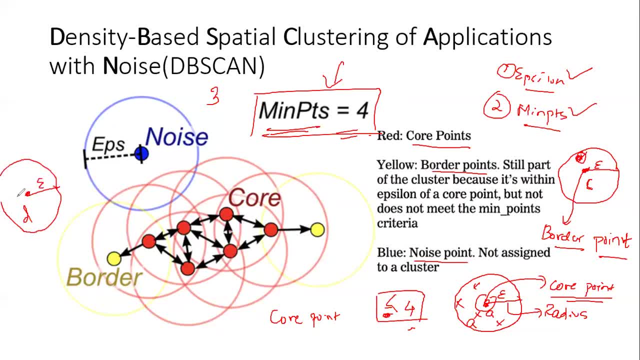 Now I have taken the epsilon radius, I have created my boundary. Now what if none of this is getting satisfied? If I don't have this minimum number of points as four, And if I don't have any core points, If I don't have any four points, then this point basically becomes a noise point. 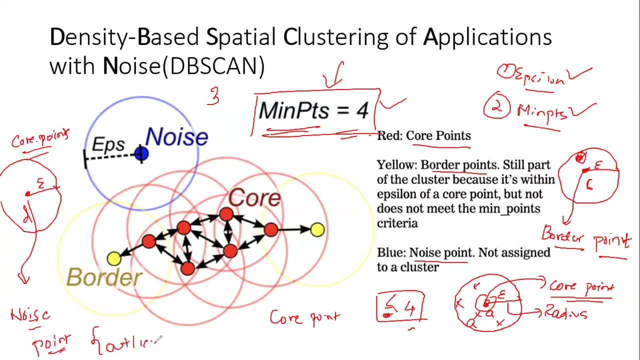 Noise point is basically like my outlier. Now this outlier is being very nicely handled by DB scan algorithm. That basically means that whenever it finds an outlier, it will never draw this kind of boundary across it. You know so it will just keep that noise point and it will never treat it as a separate group of cluster. 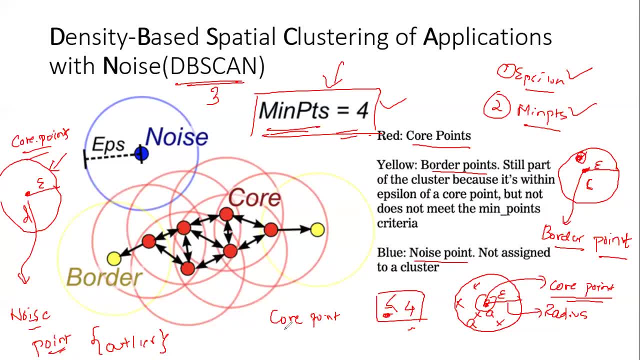 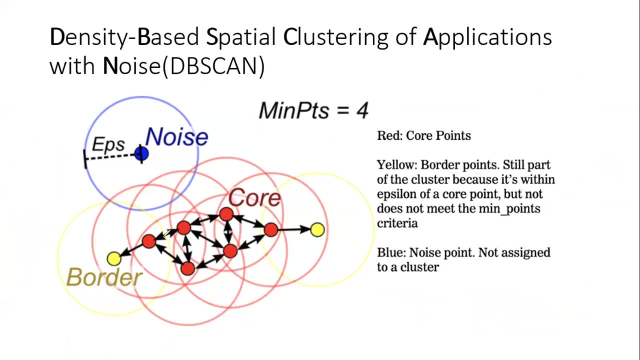 But whereas in the case of border point and whereas in the case of core point, it will be considering this kind of circular borders or boundaries, Or this is just like treated like a clusters. No, this is like a cluster. Now, you see this. Let us see this particular example that I have. 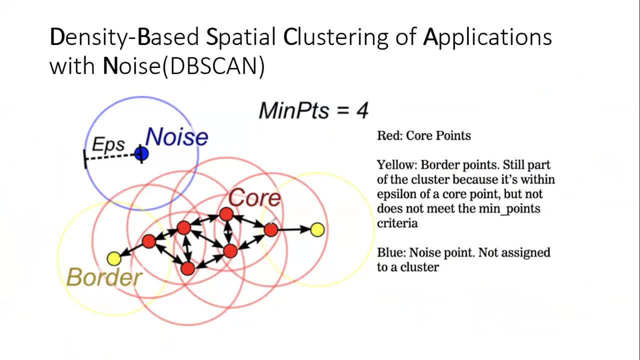 I have red points over here. You can see that this red one basically indicates that if I'm considering an epsilon value of some value And if I'm considering minimum points as four, Now suppose, if I consider this, I've drawn, I've taken an epsilon. 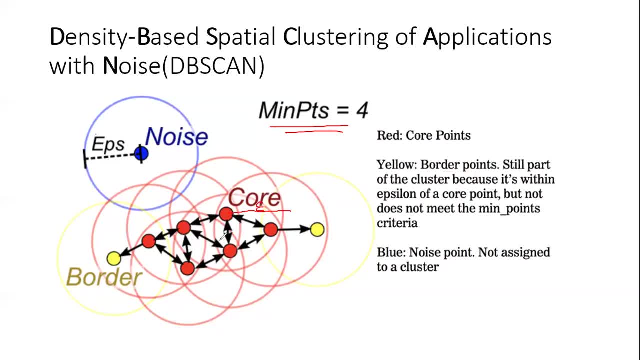 Epsilon length over here as my radius. I've drawn a circle. Now I'll go and see that at least four points are falling inside the circle. So I have one, two, three and four. So four points are actually falling inside the circle. 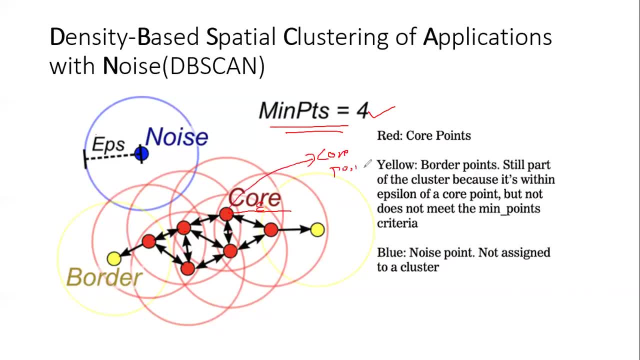 So I can consider this as my fourth point. So this, all red points, that you see, is basically my core points. OK, Now suppose tomorrow, after my model is getting trained, if I, if I, if I, if a new point comes over here, And this is basically treated as the point that belongs. 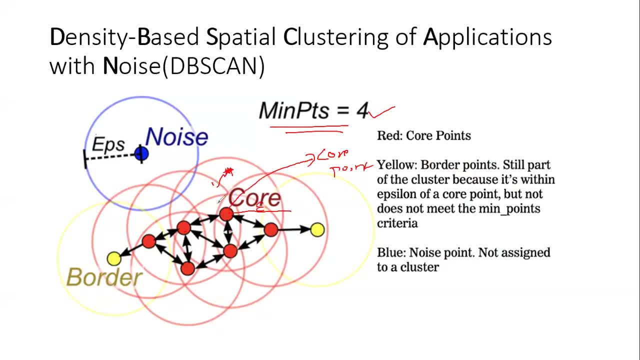 To this particular cluster, where my core point is this: Similarly with respect to all the other values. But just now, see about this particular yellow point. of this yellow point, When I draw a circle around it or a boundary along it, I don't see more than two points over here. 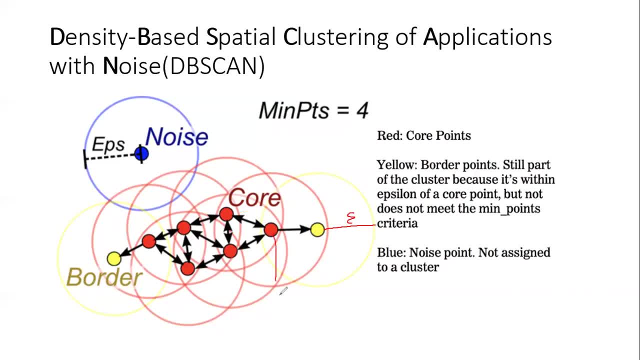 I have just one and two Right And this particular point. if it is considered as a core point, Then this basically becomes my yellow border point. So yellow, which is my border point over here. So similarly, in this case, this also becomes a border point. 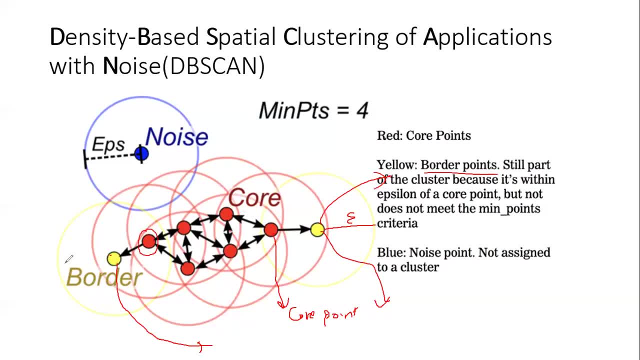 Because I have at least one, four point within this particular boundary of the yellow point. Now this is how it is actually used. You know, this whole DB algorithm, DB scan algorithm, works in this way: goes from one point to other. It tries to find out this particular value, whether it has that, but it tries to create the 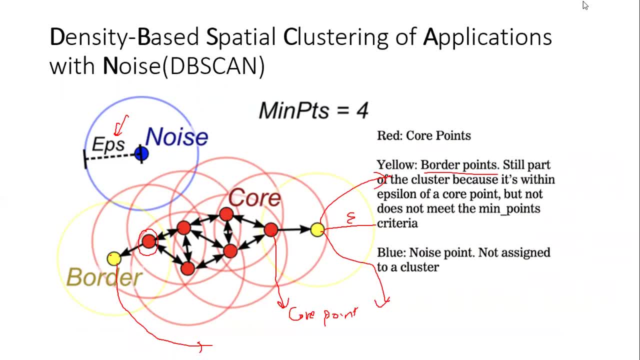 You know, it tries to create the diameter of this particular radius, that is, of my epsilon value, And then what happens is that after that, It tries to then create, you know, or try to find out, the necessary core points in this by satisfying both these conditions. 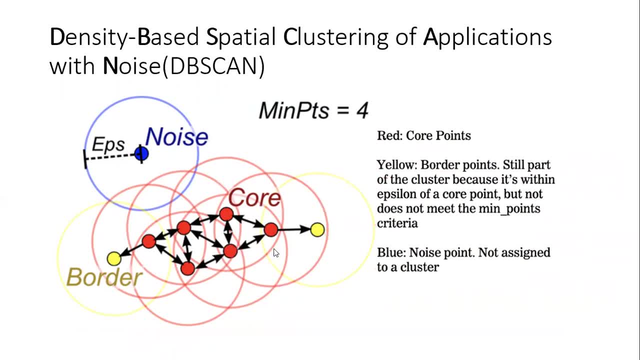 And then it classifies itself as a core point or a yellow border point. And wherever a yellow border point or a core, I mean, this yellow is basically the color. so I'm saying yellow border points, But when I see a core point I will be trying to create a cluster. 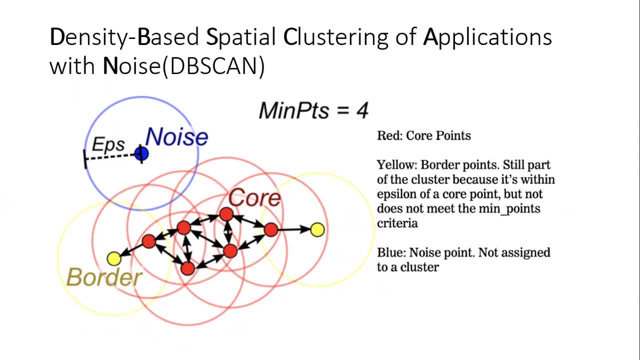 When I see a yellow point, I'll be trying to create a cluster, But whenever I find out a noisy point, I don't create a cluster. So this DB scan algorithm works very well with the noisy points, because noisy points that are never taken into a cluster. 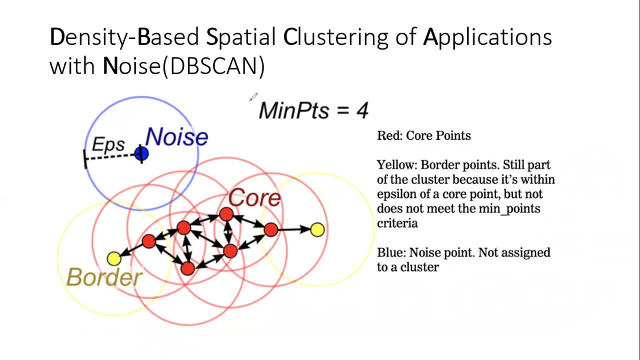 So it basically skips or does not take care of those noisy points. So DB scan algorithm works well with the noisy one, And this was an example of this. guys, Let me just go to the next slide and show you some more things about this, like how the classification happens. 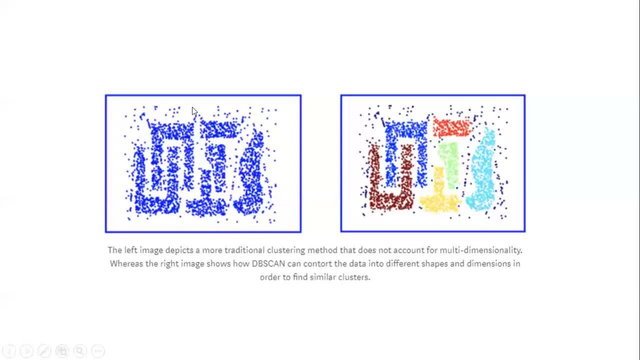 You know the left side. in the left side of the image that you see Is grouping has been done by Some other algorithm, like K-means Okay, and hierarchical mean hierarchical clustering- Okay, K-means clustering and hierarchical mean clustering, Whereas in the right hand side of the graph you can see that it is this: all clusters. has been happened with DB scan. 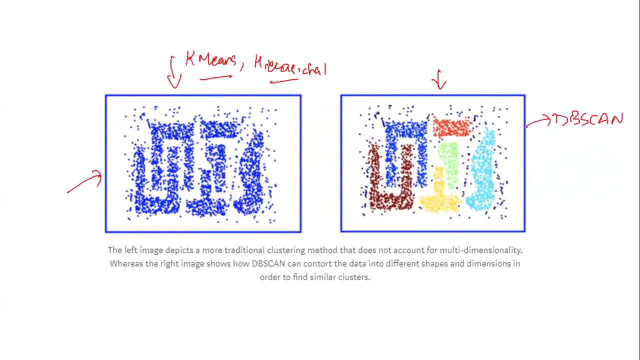 This was some of the disadvantages in K-means and hierarchical mean clustering, because when our data is actually distributed, as you know, that in K-means clustering, what we do is that we may try to make clusters of points right based on Euclidean distance, hierarchical mean clustering again. 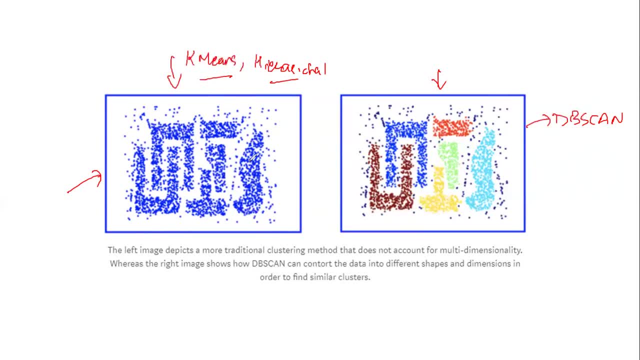 There's a Euclidean distance. Again, we follow something called, as you know, our top to bottom hierarchy to actually solve that. and similarly in DB scan algorithm- We have actually discussed about this right in DB scan You can see that it has been able to group the points very nicely. and you see this, this particular points are not group because these all are noisy points. 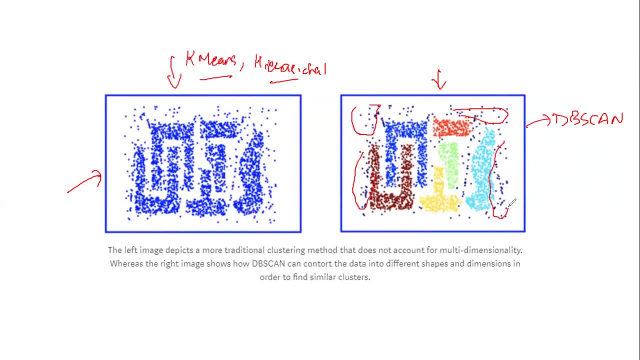 These are left like that It is. these are all left like that. you know, These are all left like that. This is all. points are left like that, But whereas the other point that you can see that it has been classified a group, very nicely. 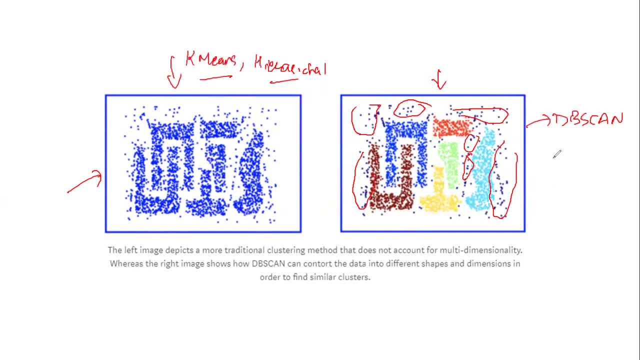 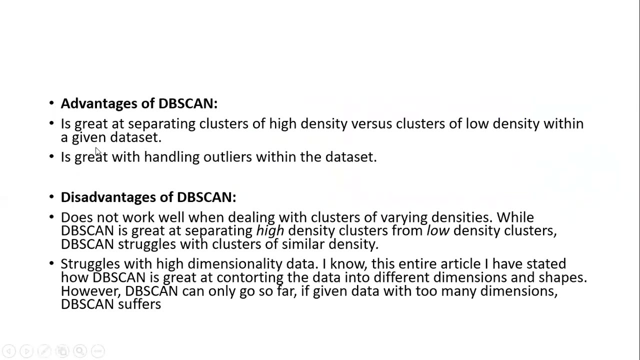 So that is the advantage of DB scan algorithm. It works very well with the noisy data. Right, It works well with the noisy data. Now, as we go ahead, guys, I'll also show you some of the advantages of DB scan. So it is very great at separating clusters of high density. 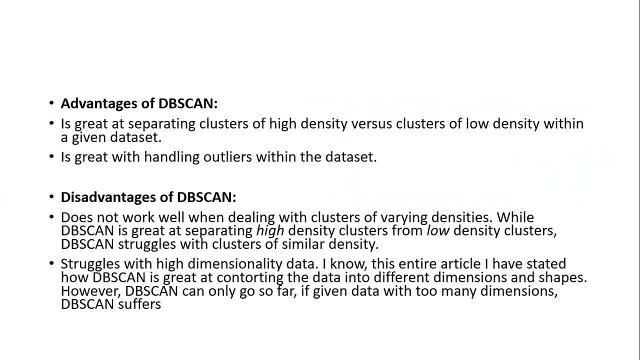 So it focuses on high density of points because we are considering two things, that is, that epsilon and the minimum points that should follow within the boundary of that, and so it It is very great at separating clusters of high density versus cluster of low density and it also defines- well defines- the noisy points, and it is also great with handling outliers. 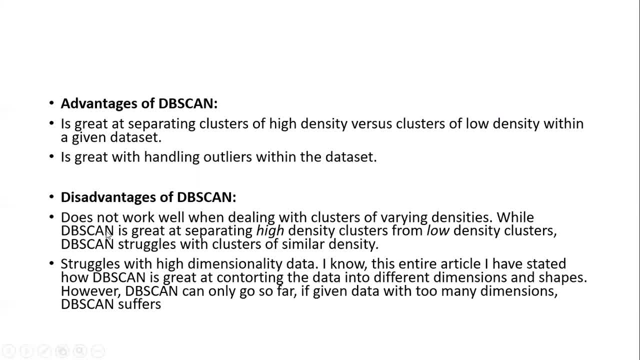 which are the my noisy points within the data set. some of the disadvantages are: it does not work well with dealing with clusters of varying densities because suppose if I have some extreme dense density in my clusters and I have, if I have less number of dense clusters? 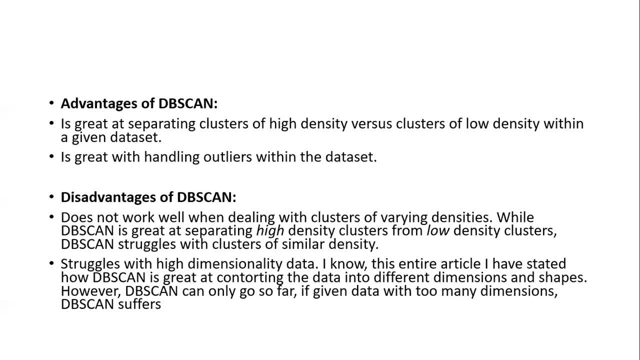 So all this kind of style, the DB scan will not work Okay. so it Also struggles with high density of data, because as the number of dimension increases, it becomes very, very difficult for grouping the data altogether by using this particular density clustering. So 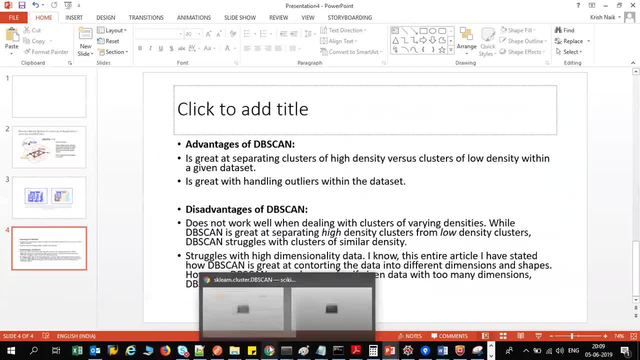 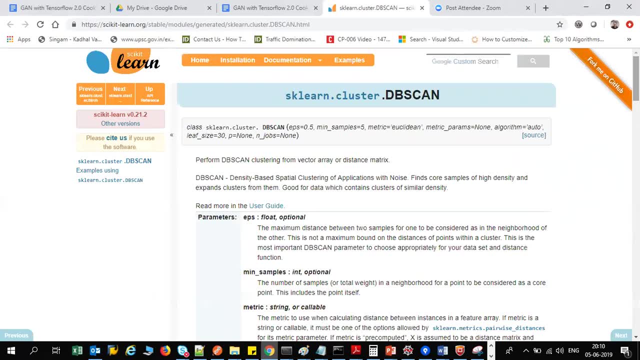 So let us, let us go and just understand how we can implement a DB scan algorithm, because I'm just going to show you a very good use case wherein will try to apply DB scan algorithm. in order to apply DB scan algorithm, guys, We will be using a library that is present inside. 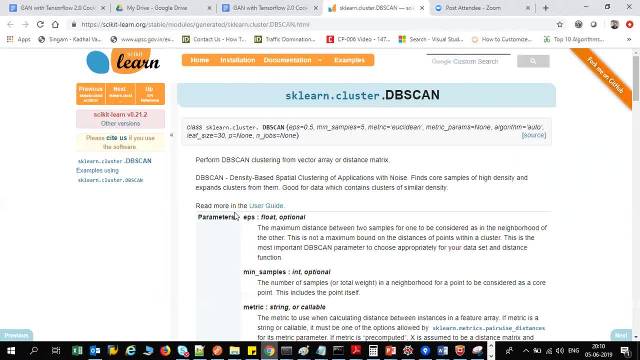 It's case. So let me just go ahead over here. You can see that we have Epsilon value, We have minimum samples, We have metric Euclidean distance, you know, and this minimum samples is basically indicating your minimum points, you know, and based on the Euclidean Euclidean distance. 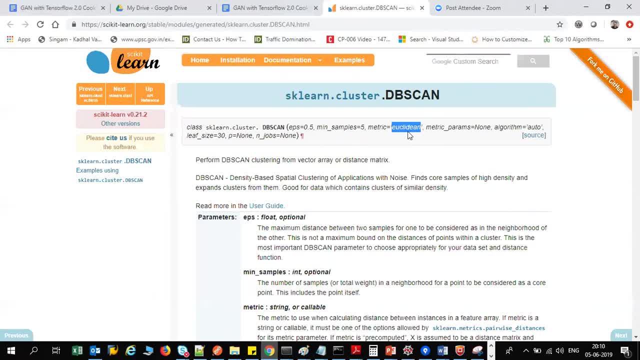 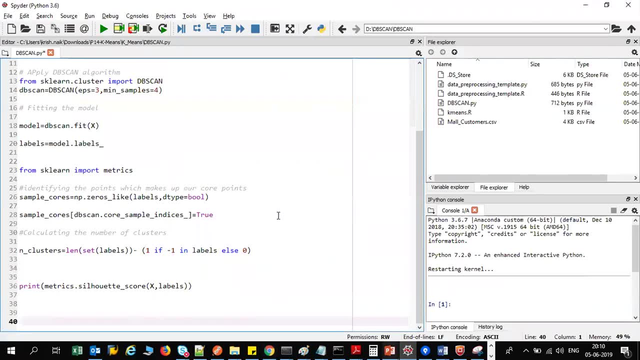 It can consider. again. There are two types of metric that we can use: either Euclidean distance or we can also use Manhattan distance. It is up to you, Okay- and how well it works with respect to this particular data. So let me just show you. 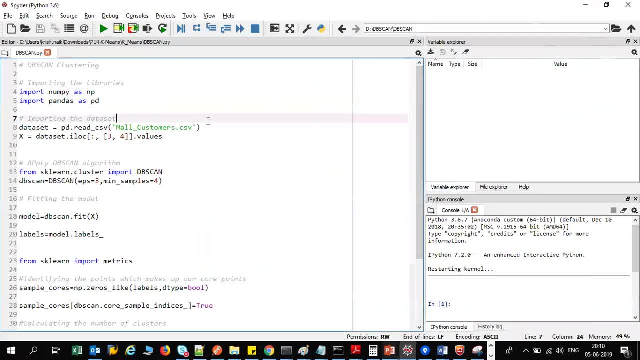 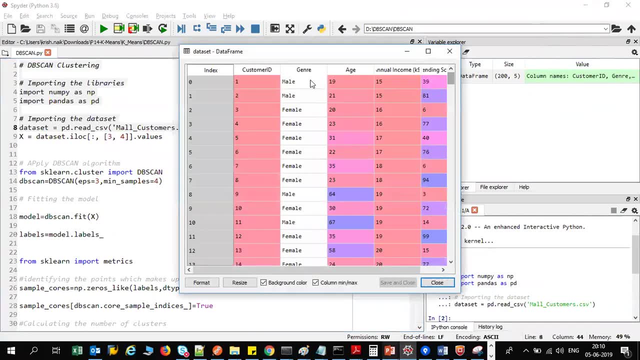 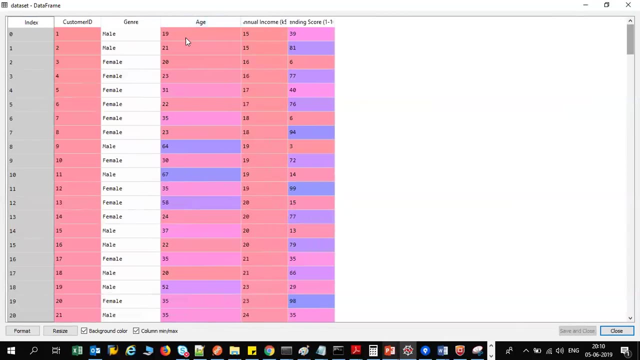 A very good example that I have for DB scan algorithm. I have a data set which is called as mall customer dot CSV. Okay, Now let me just show you the data set. Now, this particular data set. You can see that I have a lot of information like customer ID, Jen Jen Ray, or gender. 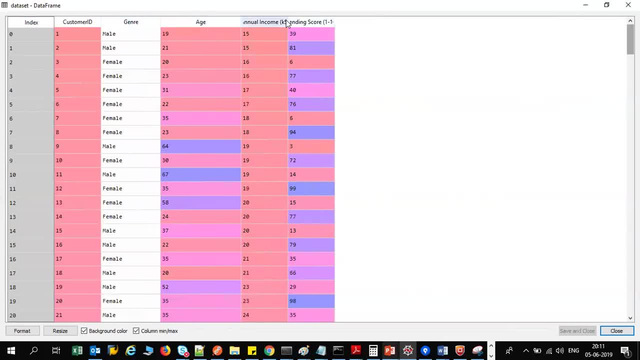 So it should be gender. It is written a gender, Then we have age, Then we have annual income, Then we have spending scope. Now what our aim should be, that I just created this problem statement that I'm going to consider: Consider annual income and spending scope. 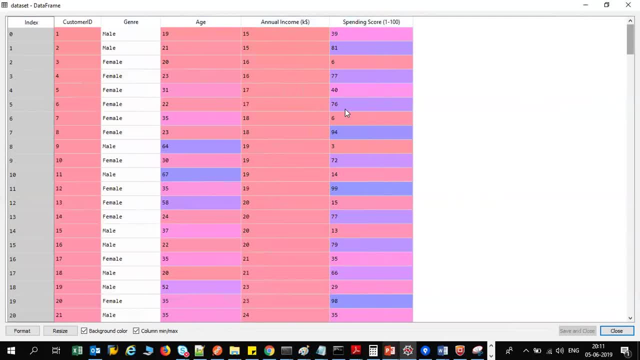 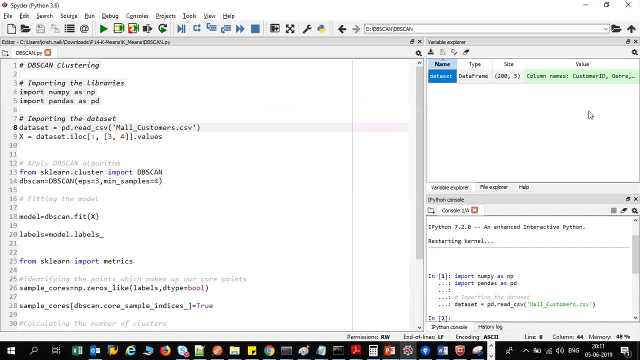 Taking these two features, I'll just apply a DB scan algorithm and, based on this density of the points, It will try to group this particular points together. Okay, So let let us go ahead and try to see. So what I have done is that I've just taken my third and fourth column. 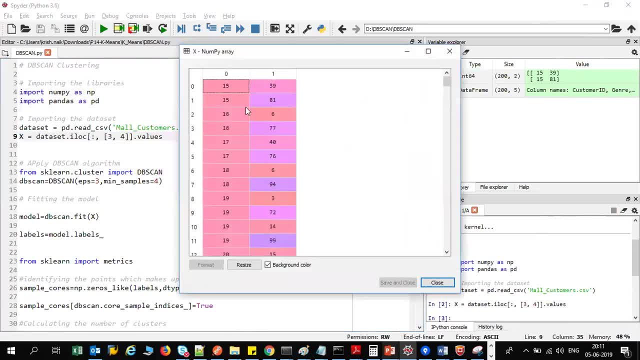 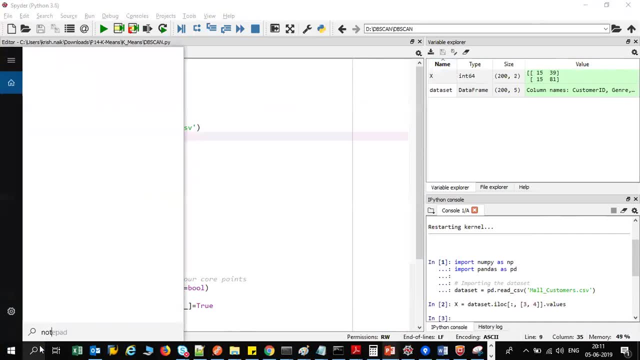 which is my annual income and spending score. So this is my third and fourth column and I've basically used a data set- oil log. So, as usual, let me just open a notepad and let me just write down the steps for you all. 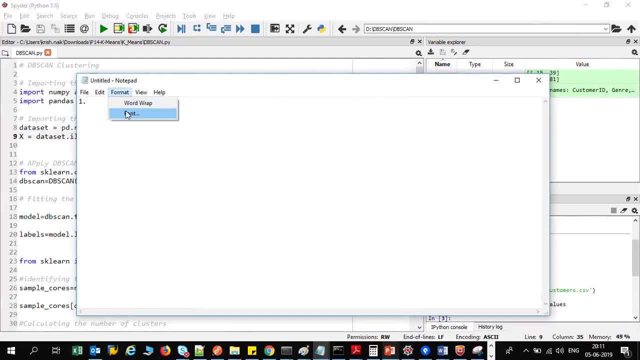 So the first step is, as usual, Let me just make the font size a little bit better and bold 16.. Oh, let us, let us go. The first step, as usual, is basically to import the data set. and, guys, this is a unsupervised machine learning technique. 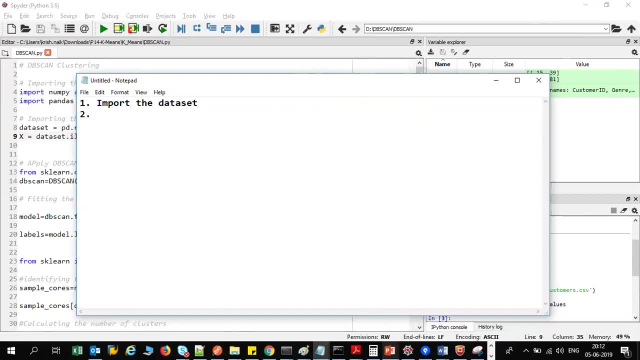 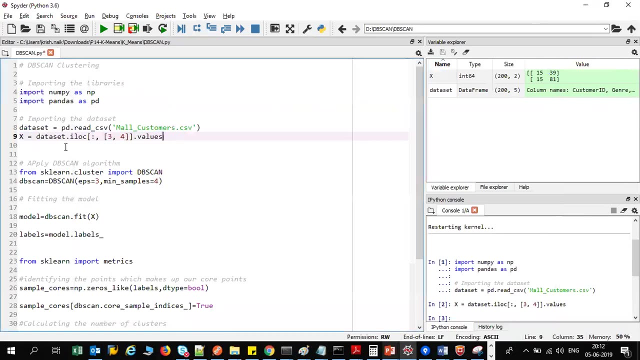 So you don't have any output in this feature, You just have independent future and finding the similarity in the feature. What we do is that we try to, based on the density scan algorithm, will try to group those into plus. Okay, after importing the data set, we'll just- and I have my independent features over here in my X. 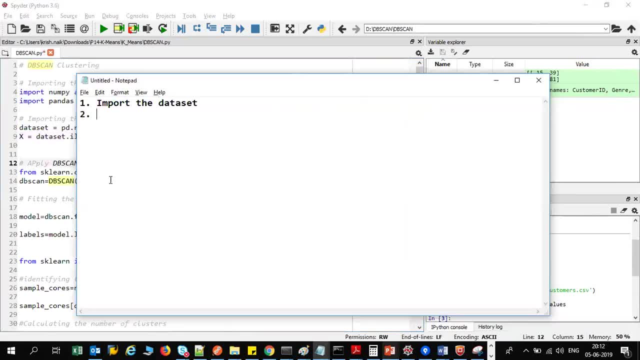 Then I will be just applying my DB scan algorithm. Now DB scan. basically, you know I have to import, import the DB scan algorithm. So, as usual, DB scan algorithm is getting imported. import the DB scan from a scale on right. So I'll just write it down so that you will always be able to remember the steps. 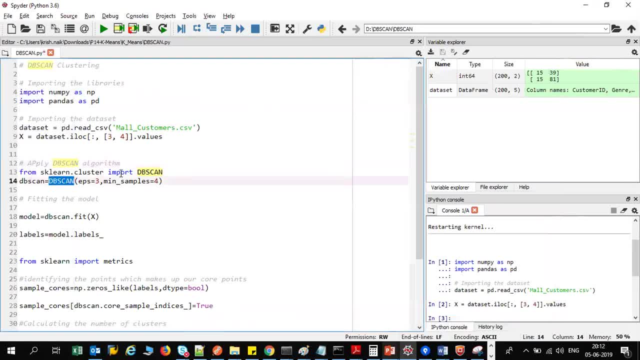 Now you can see that we have Taken the DB scan, imported the DB scan from a skill and cluster and over here DB scan, I've taken as Epsilon value as three. you know what is Epsilon, with the help of which I'll be actually creating 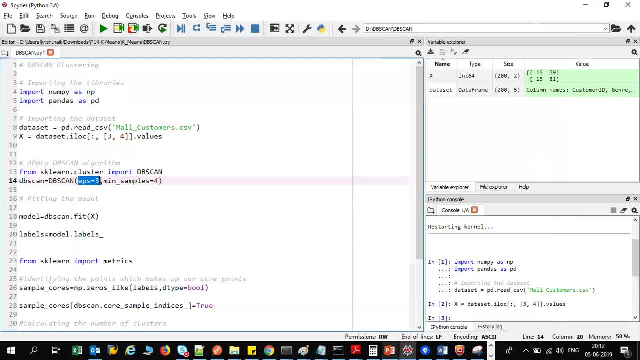 you know a radius and, based on that, I'll be creating- I'll be considering Epsilon as my radius and creating a boundary around that particular point and the minimum number of samples. I'm just considering it as for to, in order to just show you how it will work. 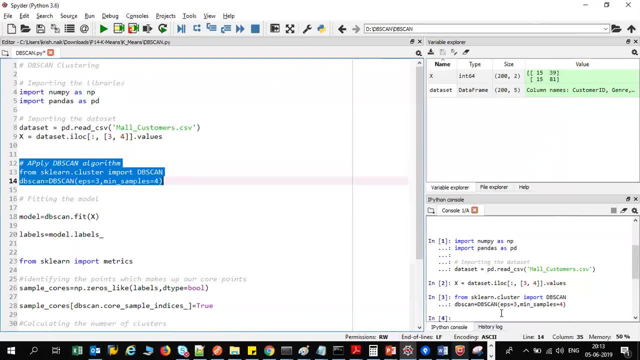 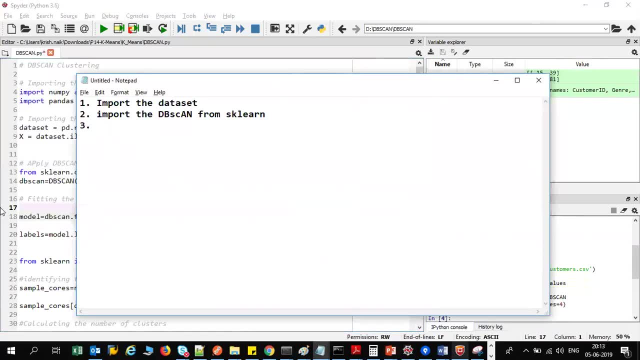 Now this is working. Now you can see that my DB scan has worked properly over here. It has got executed. Now the next thing is that I'll be fitting the model you know. so, as usual, my third step is basically fitting the model you know. 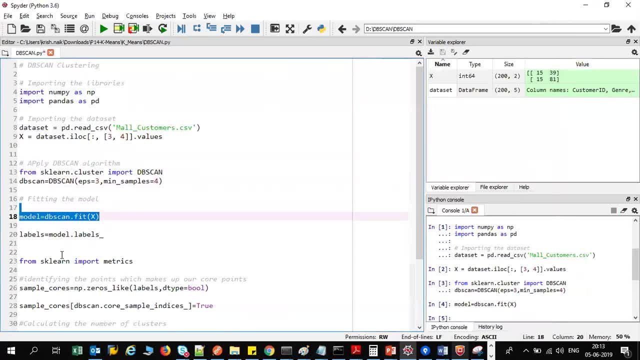 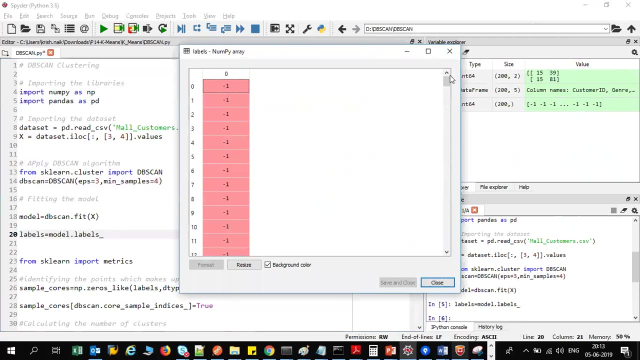 that basically means that my training will start over here. Now, this is fine done. as soon as I do this, after doing the fit, If I say model dot labels, I'll automatically get all the labels. You can see that now. my labels is like this: now, from the labels, that basically means that how many clusters of groups I'm getting it? 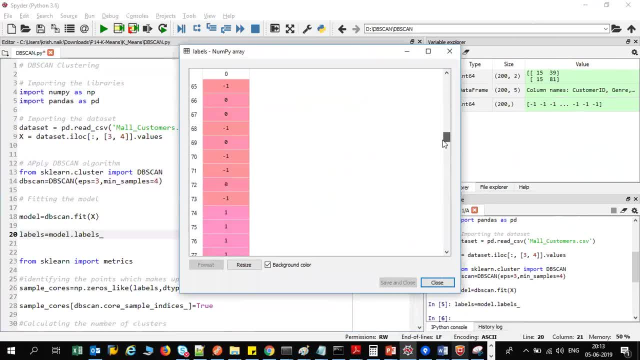 You can see that over here There are a lot of values which will have minus one. Okay, Can you just imagine what this minus one will be? Well, there are one zeros minus one. You can see one over here: two, three, four, five, six, seven, eight, and remaining all our ones. 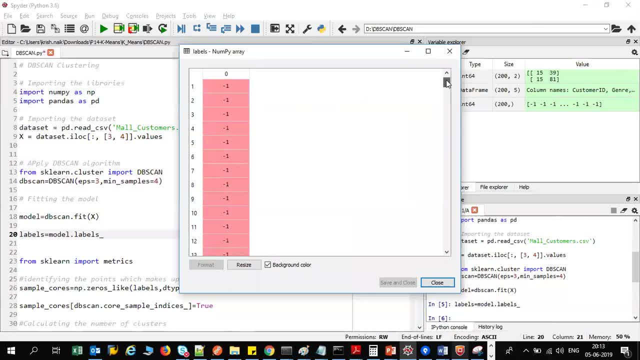 Okay, so zero to one. I have a lot of this. understand this minus one basically indicates that these points are the outliers Okay, and it did not fall in any of the clusters, Whereas other points. you can see that it is starting from zeros than ones. 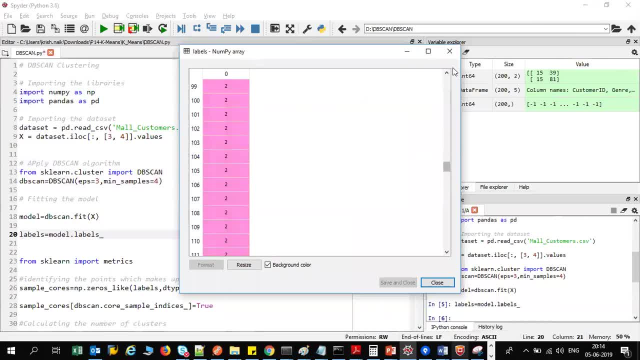 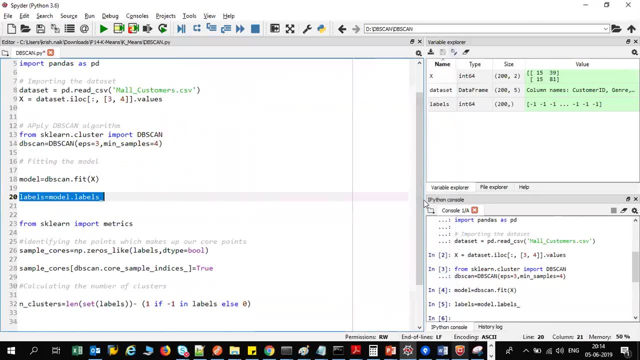 Then these are basically my zero cluster, First cluster to cluster. So many groups of clusters are there? Now what I'll do is that I will try to find out how many unique groups are there. Okay, So for that, first of all, I'll just- I'll just create a array, array by using numpy, where I will consider everything as false. 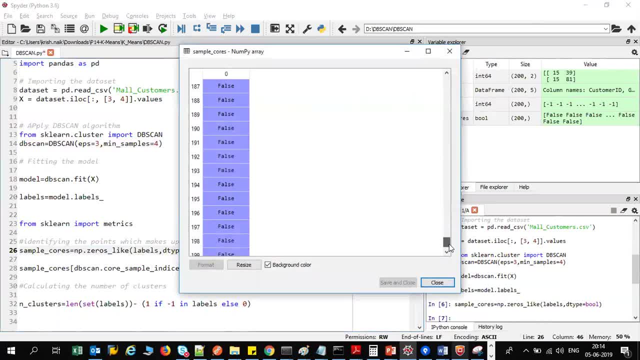 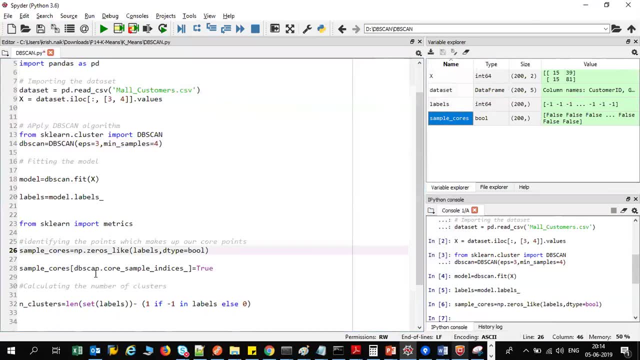 So this is the code to do that. You have everything as false right now. Now what I'll do: I'll compare this sample underscore course and labels and wherever these label values are true. So suppose if I just write DB dot core underscore, sample underscore, indices. 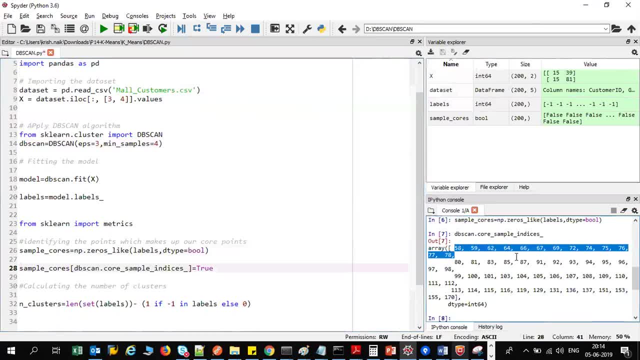 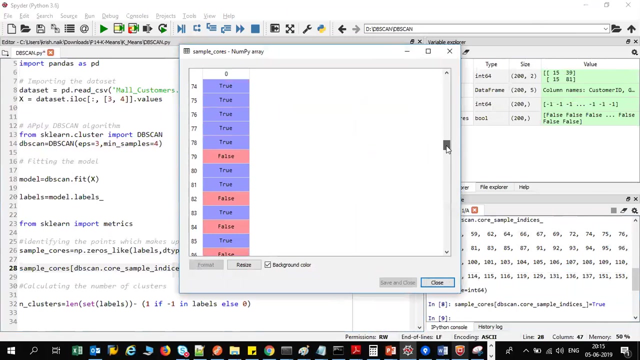 This basically indicates that on which all index, which all index, I'm having a different value. I'm having a different value which is like a group, you know, apart from minus one. Okay, So what I do is that I'll take all these indexes and I'll make it as true, because this basically indicates that this many from the sample underscore code, whichever all false remaining, all are basically my groups. 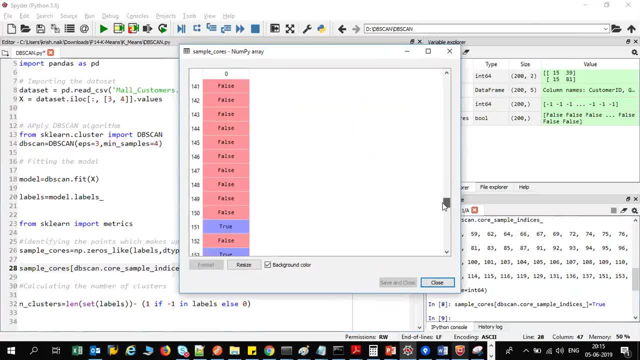 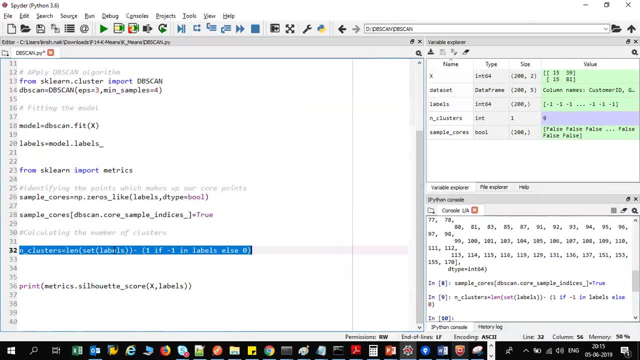 Define Different different groups So you can see that all the true values are there. Then I'll just calculate the number of clusters. If I do that, I just use that length, length of set of labels. minus this, You can see that my total number of clusters are nine. not be considering minus one as my cluster, because minus one is the noisy points, the total number of cluster.